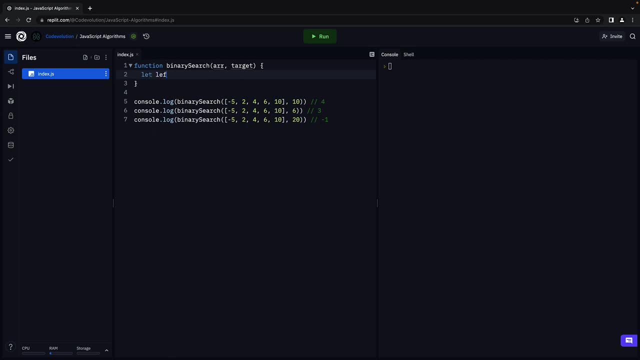 of the array, So let left index is equal to zero, since array index starts at zero. So let left index is equal to zero, since array index starts at zero. Since array index starts at zero, let left index is equal to zero, since array index starts at zero. 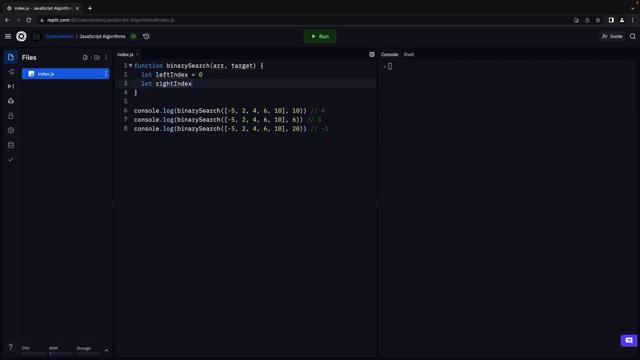 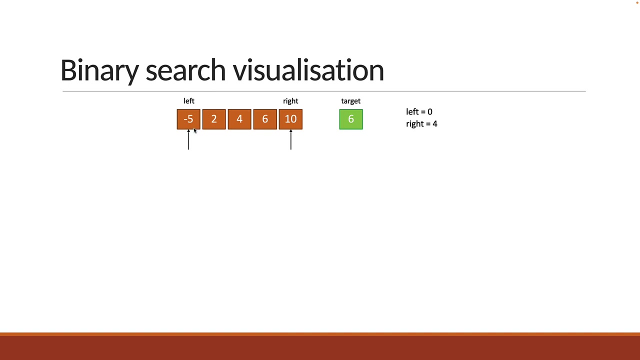 0, and let. rightIndex is equal to arraylength minus 1.. In our example, leftIndex is equal to 0 and points at the first element minus 5, and rightIndex is equal to 4 and points at the last element, 10.. 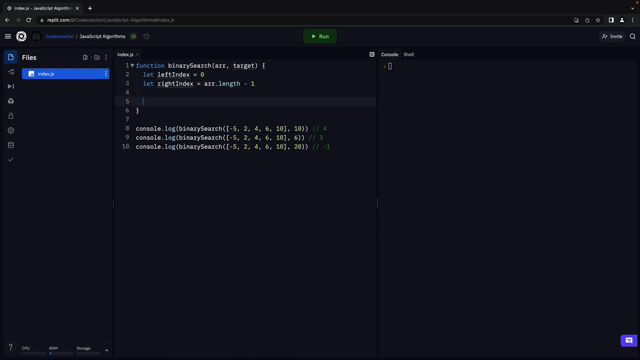 The next set of operations. we repeat: as long as the array is not empty. So we add a while loop with a condition that runs the loop as long as the leftIndex is less than or equal to rightIndex, while leftIndex is less than or equal to rightIndex. 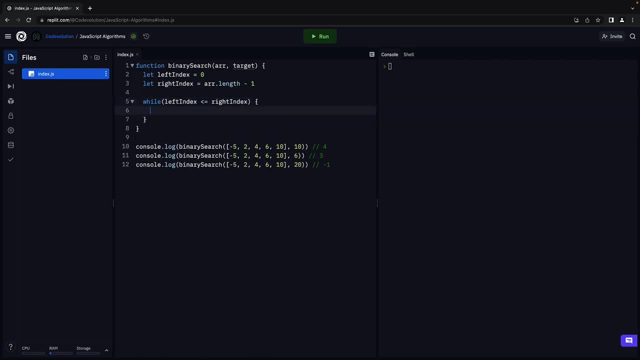 Now in each iteration we find the middle element. So let: middleIndex is equal to leftIndex plus rightIndex divided by 2.. If we have an even number of elements, middleIndex might be a decimal. So we use mathfloor to return the lower integer value. 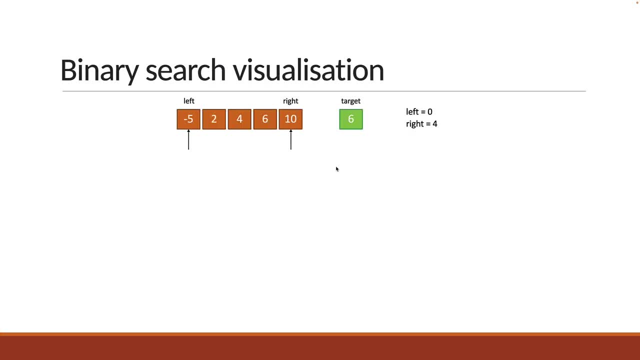 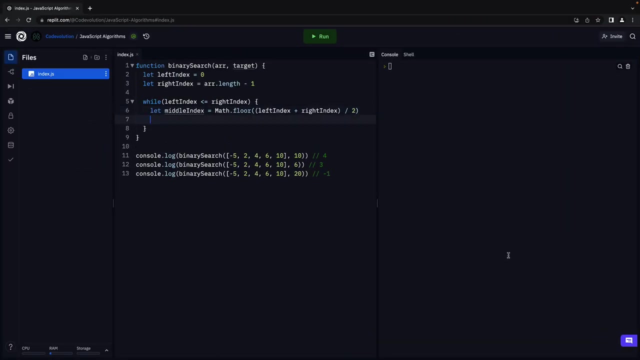 In our example, this would be 0 plus 4 divided by 2, which is 2.. Left is 0,, right is 4, mid is 2.. The middle index points at element 4.. We now check if target is equal to the middle element. 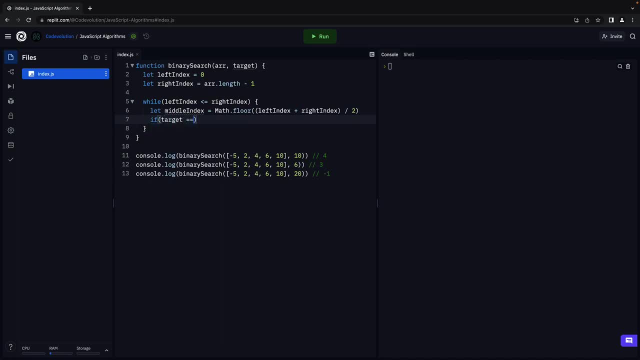 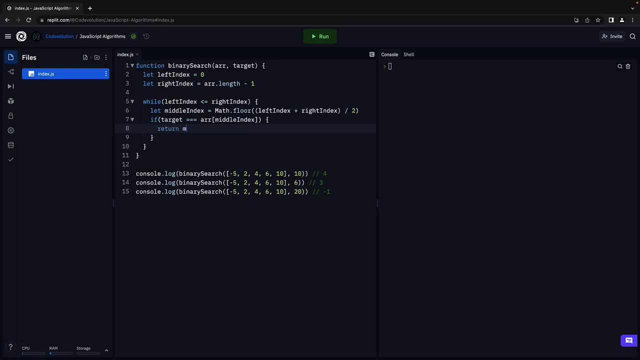 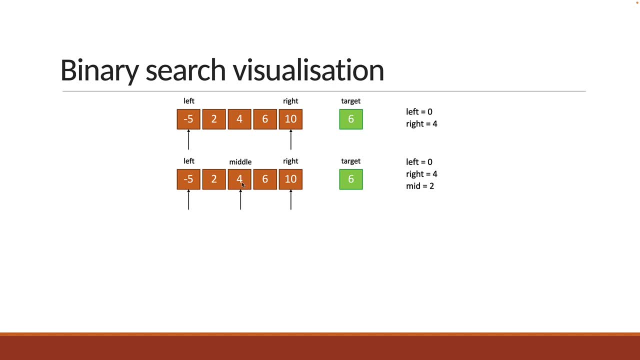 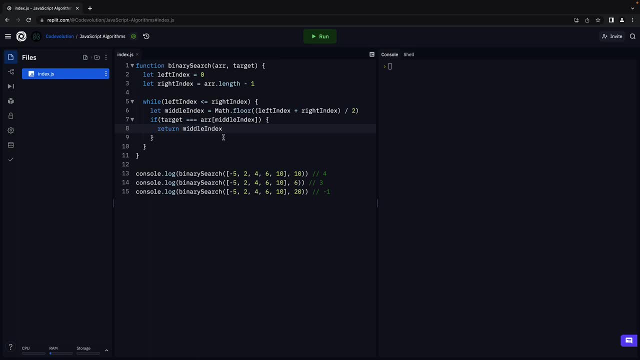 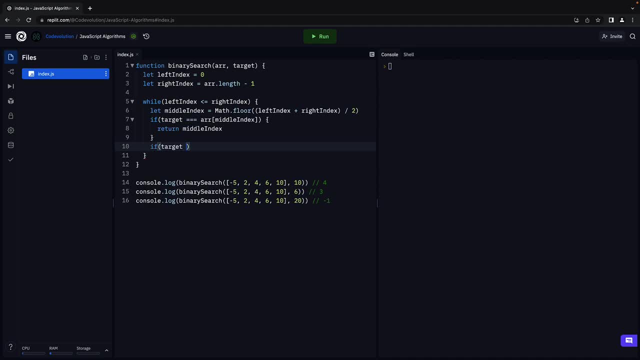 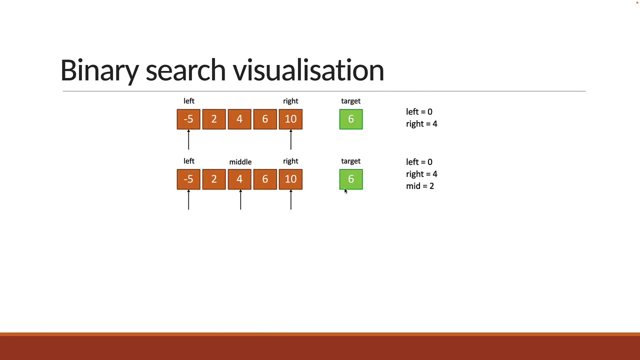 If target is less than the middle element. so array of middleIndex: we change the right index to middleIndex Else, That is, if target is greater than the middle element, we change left index to middle index plus 1.. In our case, the target element 6 is greater than the middle element 4.. 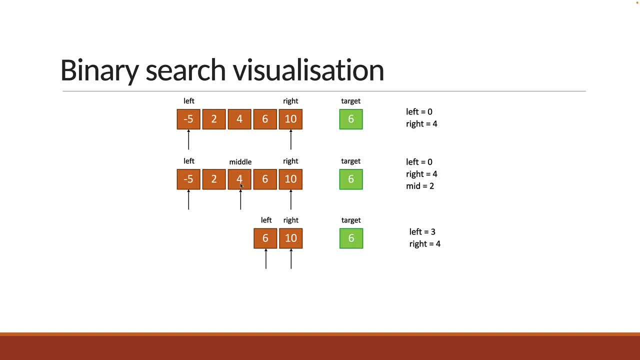 So we change the left pointer to point at middle index plus 1. The left now points at element 6 and right continues to point at element 10.. The left index is 3 and right index remains 4.. And remember, we do this because the array is already sorted. 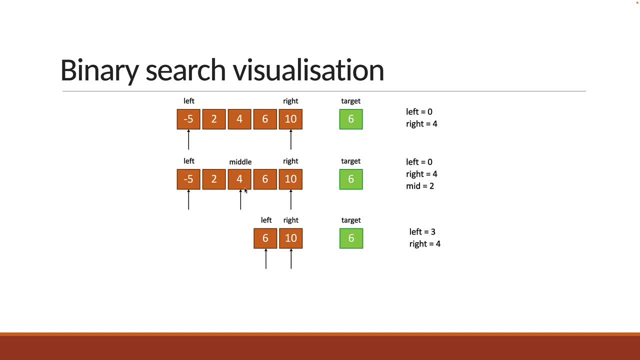 We know that 6 has to lie to the right of the middle element, since 6 is greater than the middle element At this point in time. since left is less than or equal to right, that is, 3 less than or equal to 4, we repeat the while loop. 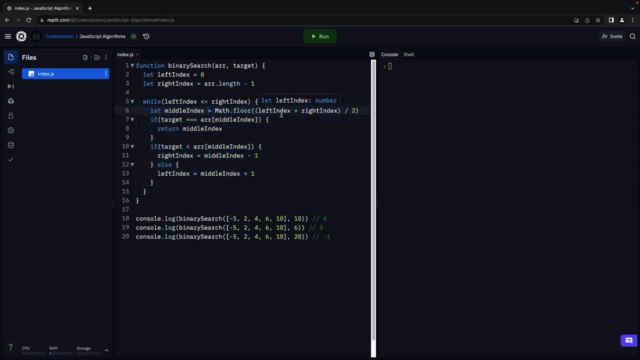 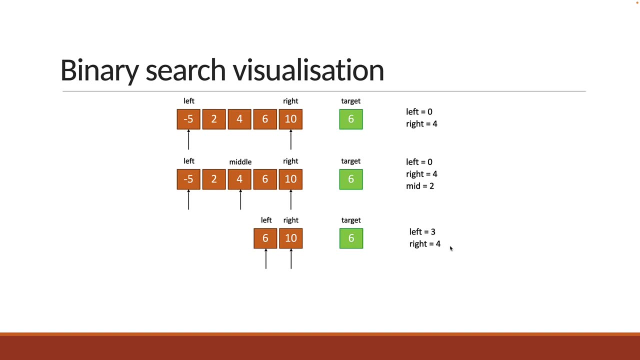 We calculate the middle index again, which is left plus right divided by 2.. So 3 plus 4 divided by 2. That is 3.5, but matfloor will convert it to 3 and middle index is now 3.. 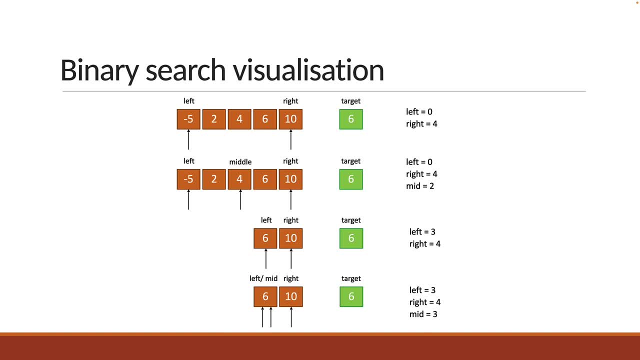 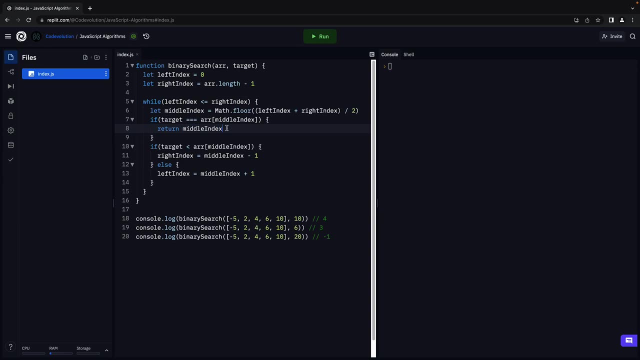 We check if the element at the middle index is equal to the target element. 6 is indeed equal to 6. And we return 3 as the middle index position And that middle index is the position of the element in the array. Our code will return from binary search function. 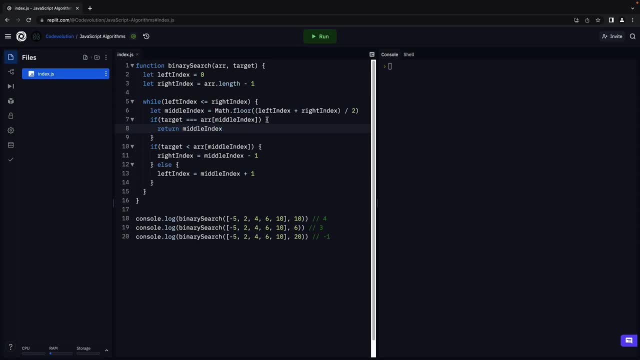 Of course, if the element is not present, Eventually, Our while loop Condition fails. In that scenario, we return minus 1.. This indicates the element is not found. This is pretty much your binary search algorithm. Let's verify by running the code. 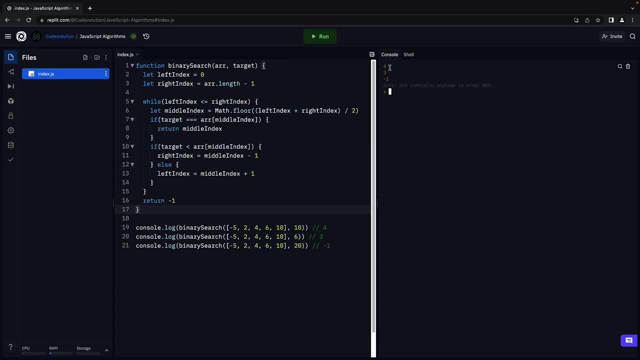 Click on run And we see the three values corresponding to each function call. Our code works as expected. What I would like you to do is take a pen and paper, trace the function. execution for this array And target is equal to 10.. 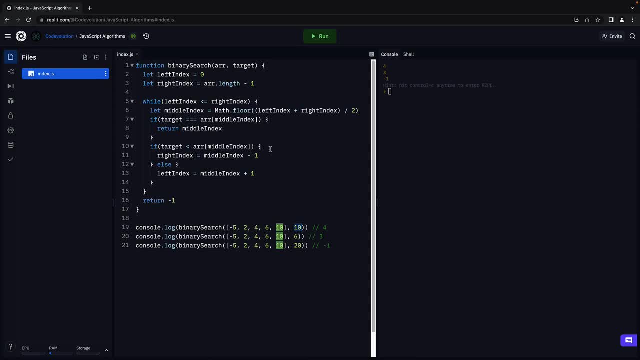 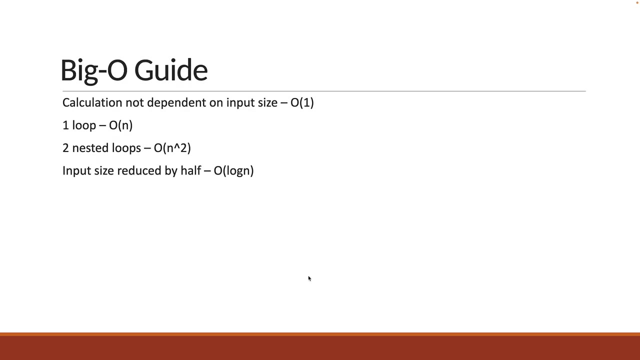 That will improve your understanding of the code we have written. Alright. Next it's time to determine the big O of our binary search function. Pause for a minute and determine the big O. Here is the cheat code. Here is the cheat code. 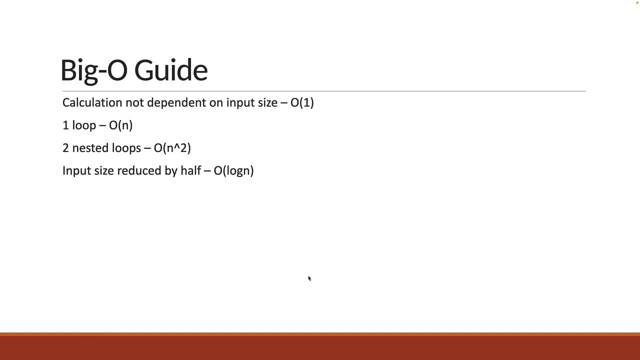 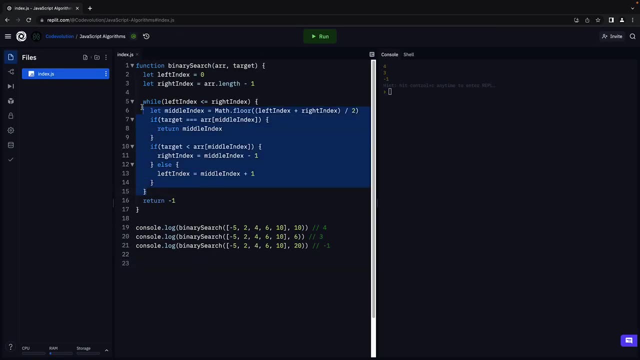 Here is the cheat sheet which can be used as a guide. Pause now. or let's estimate the big O together. Our function contains one while loop, But the detail is inside the while loop. In every iteration we reduce the input size by half. 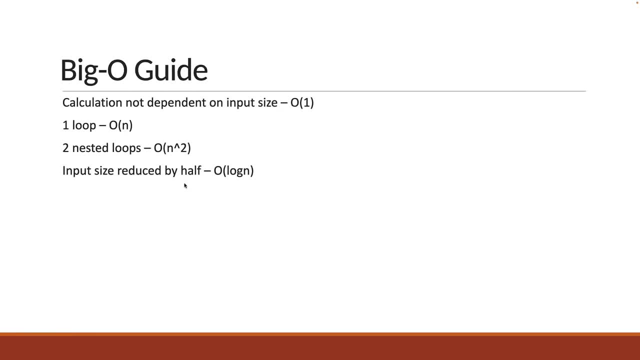 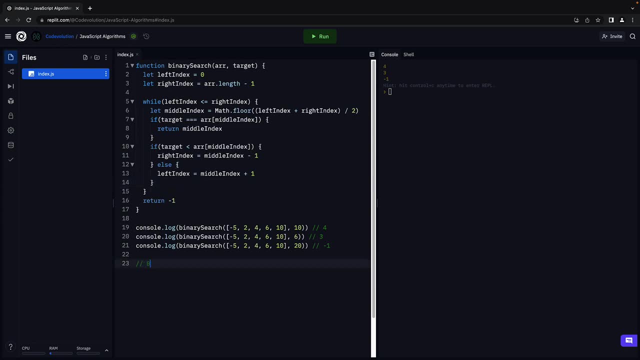 So the time complexity of our function is O of log n and not OO. N here refers to the size of the array. The number of instruction executions increases as n grows, but not by the same amount. Time complexity is logarithmic and not linear. 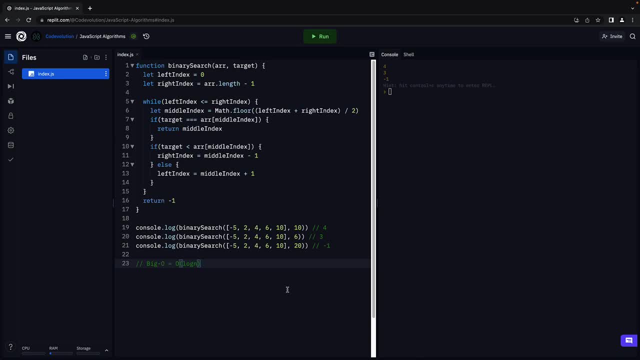 Alright, In the next video let's take a look at the recursive solution to binary search. Thank you for watching. See you in the next video. Bye, Thanks for watching. Make sure to subscribe to the channel and I'll see you in the next one.